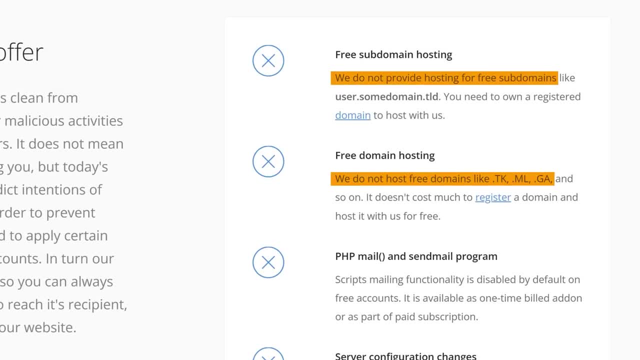 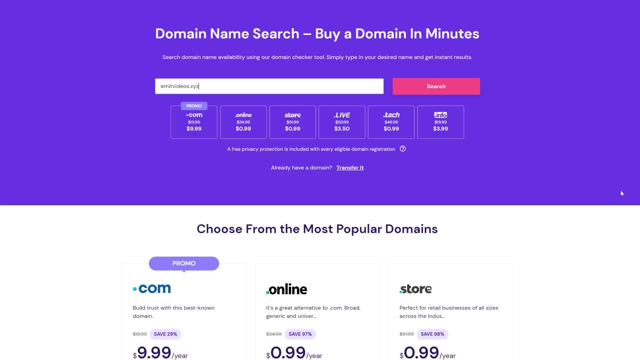 Can't add a subdomain, and you can't add a free domain as well. It must be a legitimate one, otherwise the hosting service won't work. If you're really looking to save, I recommend grabbing one of the 99-cent domains from Hostinger. 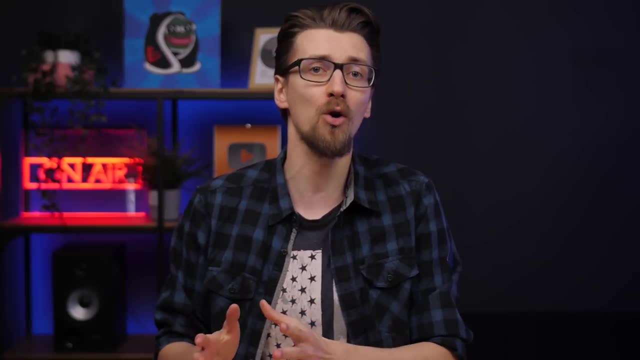 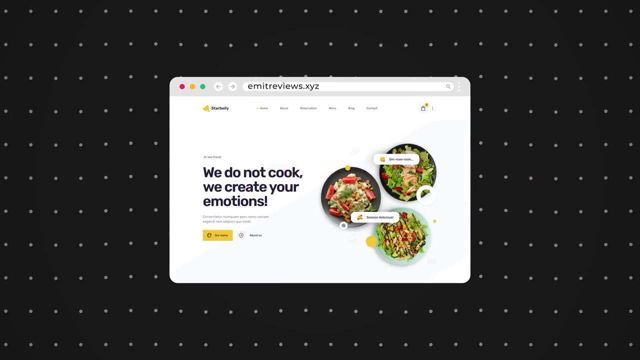 like xyz or online. They work here with no problems and they only cost you $1 for a full year. Once my domain was added, I managed to upload a backup website that's quite heavy- Around 400 megabytes of content. 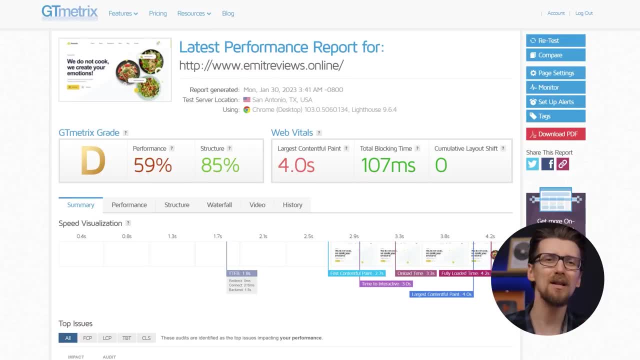 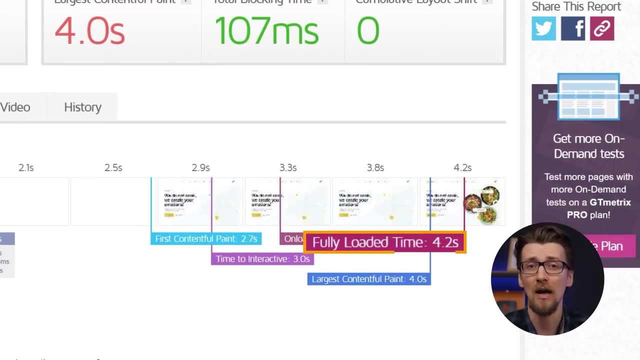 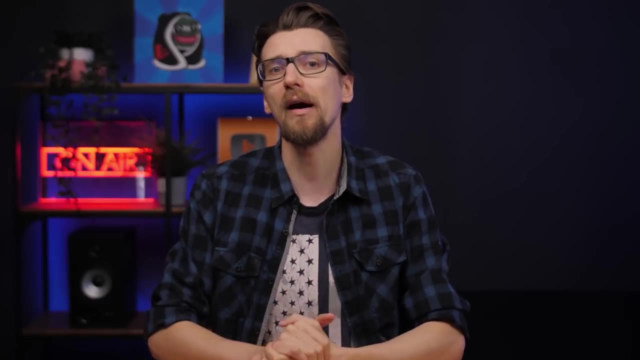 with lots of pictures and animations. The performance is nothing special kind of what you would expect from free hosting. Full load time of 4.2 seconds mean it's around four times slower than your average paid option, even the cheapest one you could find. 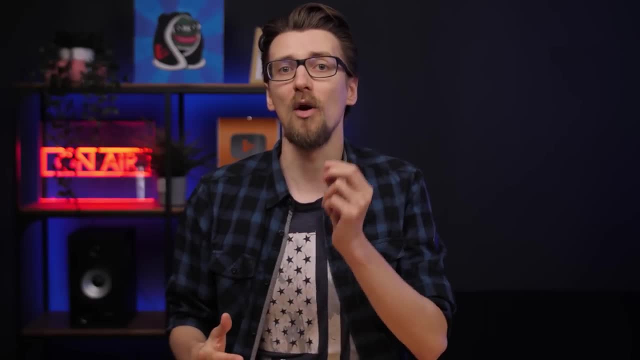 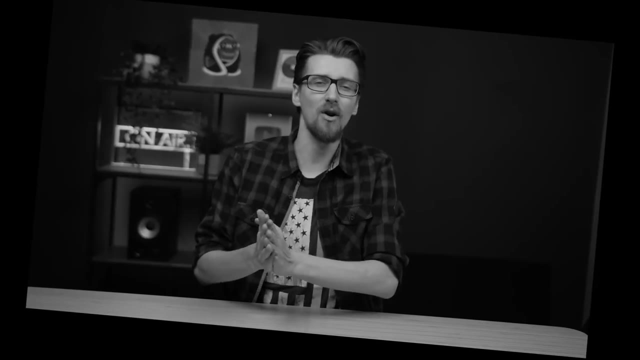 And I wasn't able to set up Lightspeed to work properly, so this is an unoptimized website. Theoretically it could be faster with some more time put into it, but this is free hosting and I don't think it would be that much better. 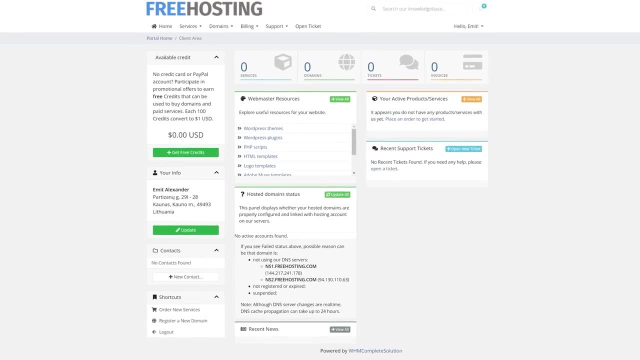 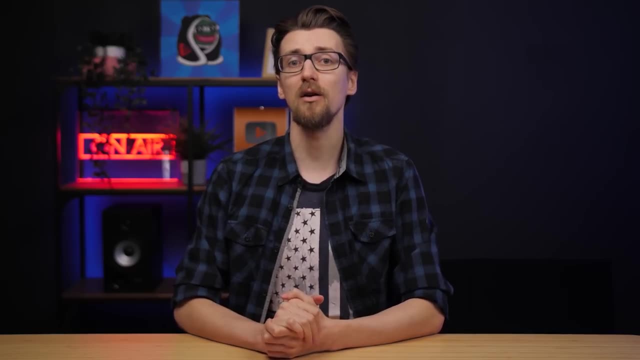 On the bright side. there are no ads, no banners on the freehostingcom website, the control panel or even your site. The way they seem to be making money is from selling these add-ons like mailboxes and subdomains. 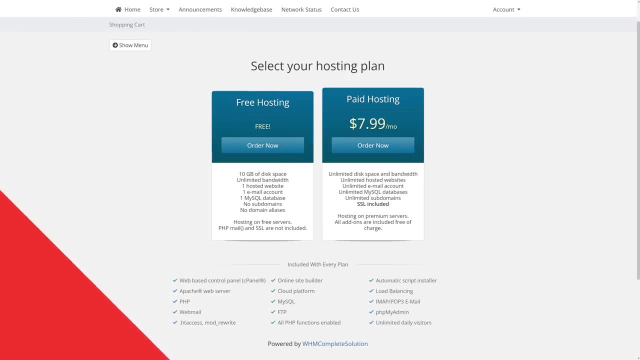 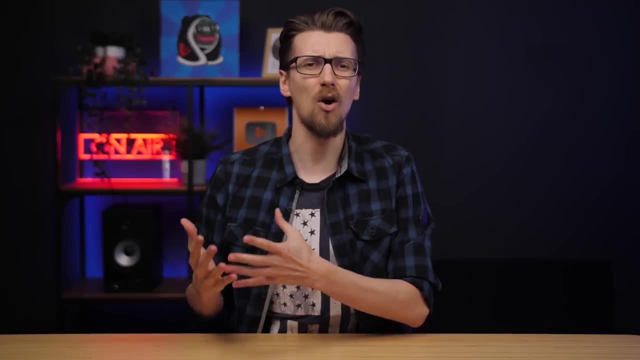 for quite ridiculous pricing, I might add, And they even have a paid plan for $7.99, which again is quite high. Never buy these paid options, because for the price of one add-on you can actually get premium web hosting. 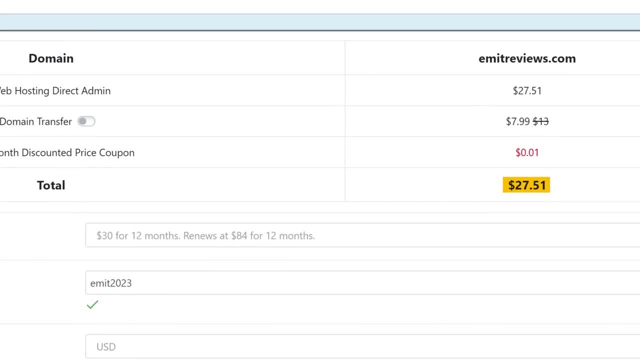 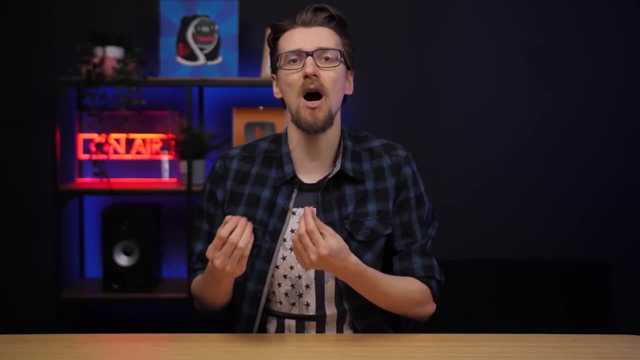 from InterServer for 12 months straight, So these add-ons obviously quite a bad deal. What really helps freehostingcom, though, is the fact that there are no sketchy clauses in their terms of service, apart from the fact that they do collect information. 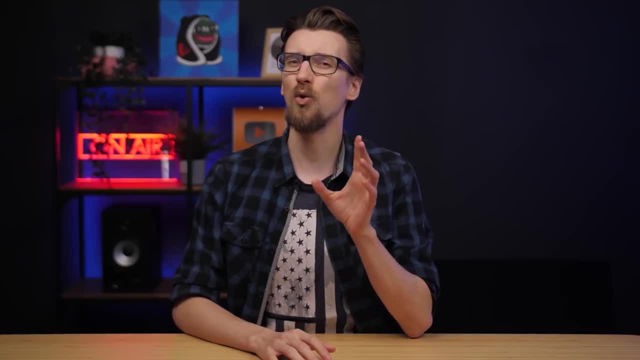 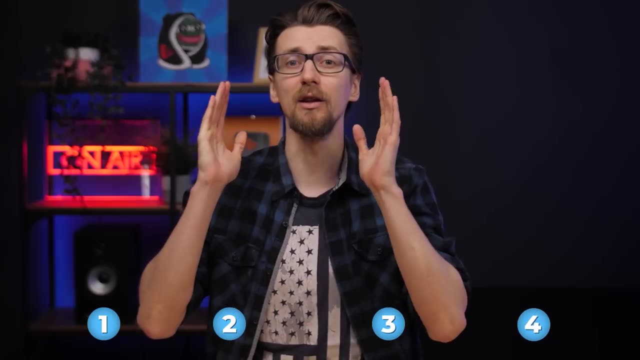 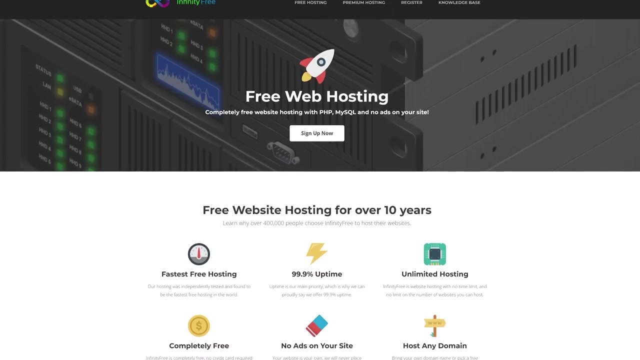 about you to provide their service, which is quite standard stuff. most businesses do this. most businesses have this in their terms of service. Now, what's completely not standard is the terms of service of Infinity Free, While they also offer free hosting with more free perks like SSL certificates and cPanel. they pretty much reserve the right to sell your data and your website's visitors' data, like payment information, emails, IP addresses, names- pretty much everything- for various marketing purposes, like surveys, demographic studies, et cetera. This is pretty much how Infinity Free makes money. 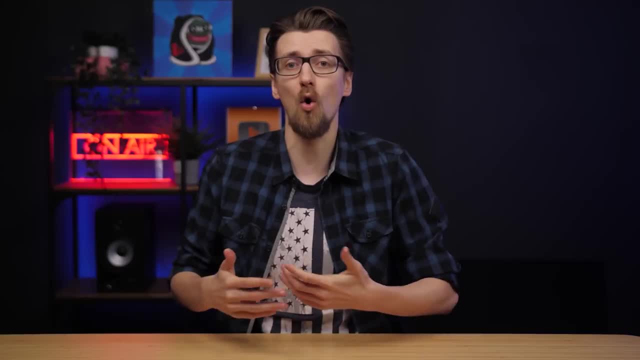 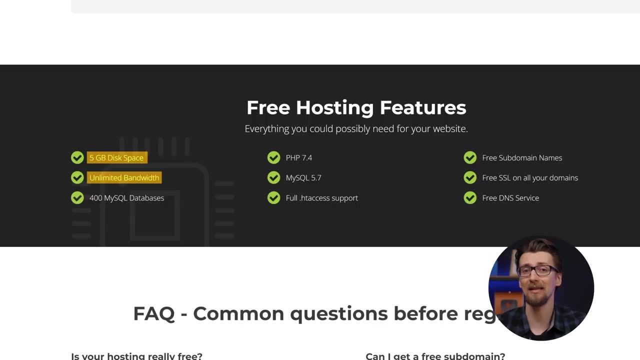 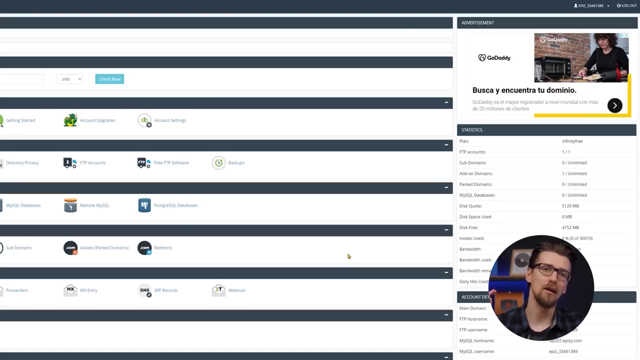 And for that you get free hosting that requires no credit card or verification. There are no limits on storage or bandwidth, or even simple functions like add-on domains and subdomains. Everything's unlimited. But again, you'll see ads everywhere: In the control panel, on the main page and in the menus. 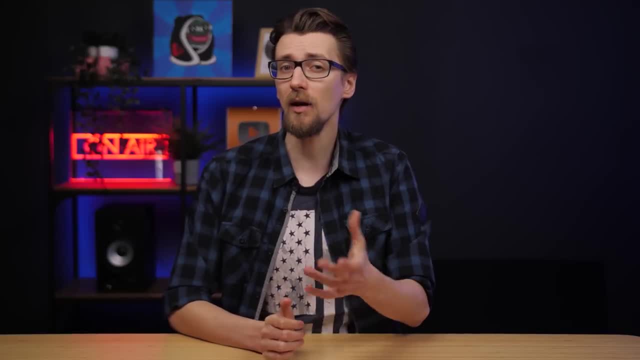 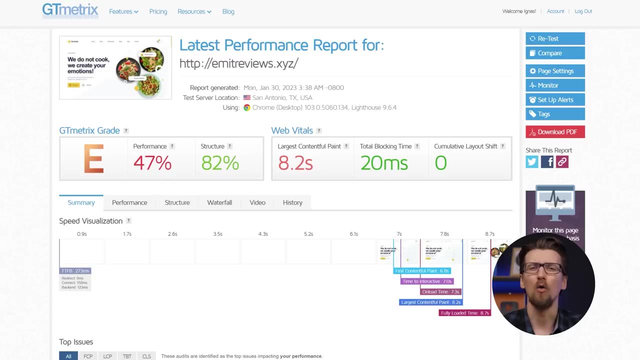 Just like with the previous provider, I've created a website quite easily using the automated WordPress tools provided and managed to upload the same website backup to test the performance: Oof 8.7 seconds full load time- two times as slow as freehostingcom. and eight times as slow as a standard paid provider. A funny thing is that when you're activating your account, they show you this warning that if you do not accept email offers from them, they might deactivate your account. Quite a cheap scare tactic. 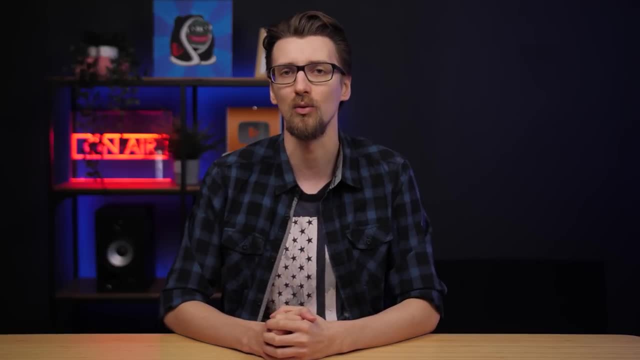 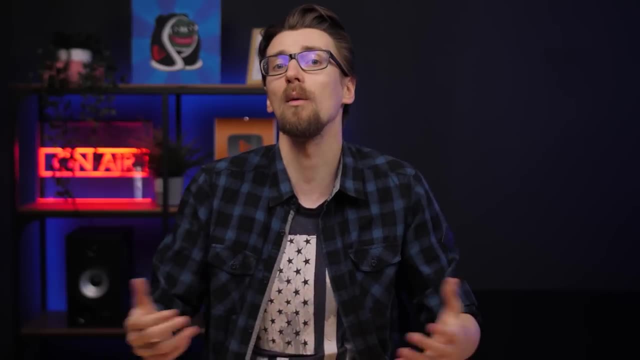 please don't ever accept this. They have no legal right to do anything about it. But moving on Infinity Free will give you a better, more authentic experience of how web hosting works, because they're using industry standard control panels and tools and they don't have any limits. 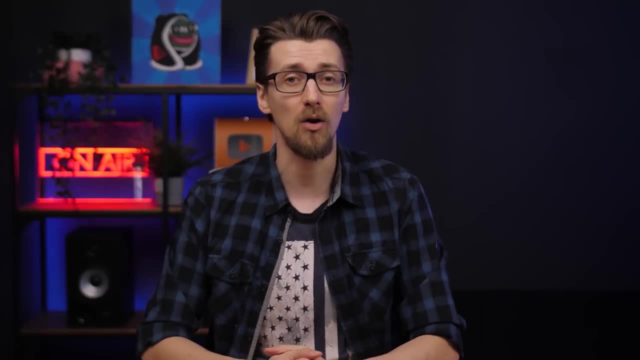 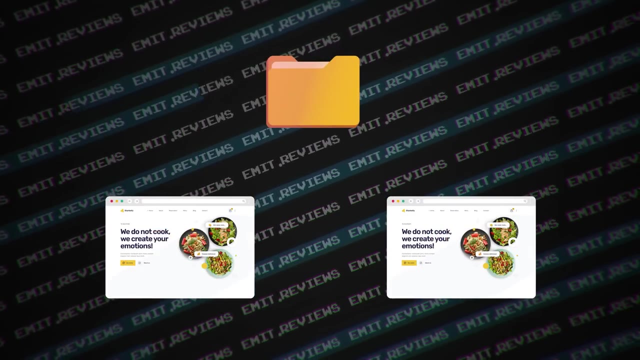 So if you're looking to learn, this is probably a better option than freehostingcom. Anyways, up to this point, I was able to load my test websites into these free providers via backup functions. absolutely no problem- Not with 000webhost. 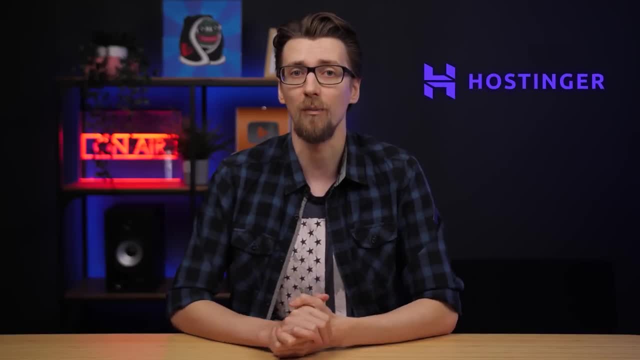 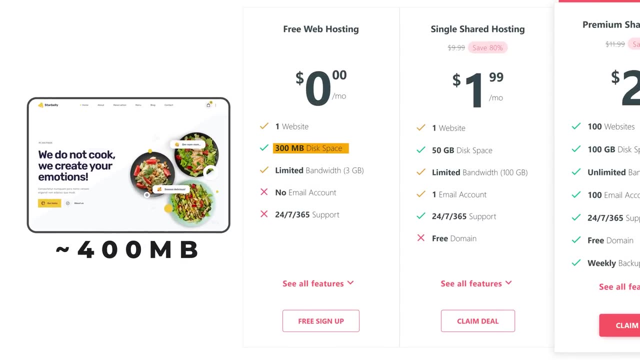 000webhost is a free provider that's part of Hostinger, a larger web hosting company. However, they only give you 300 megabytes of space and my website takes up more. Actually, after installing WordPress using their automated tools, I'm already up to 150 megabytes. 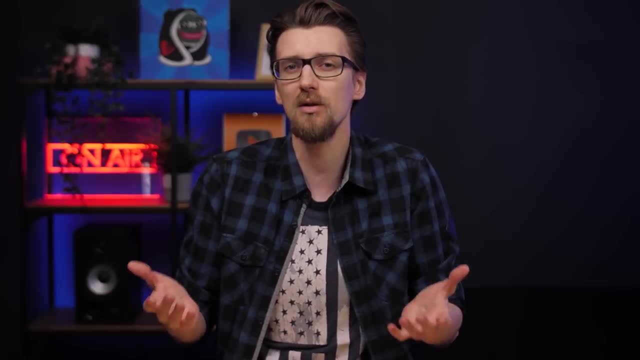 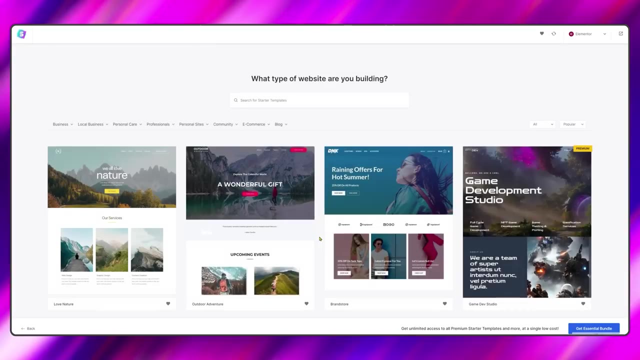 So I don't have enough space to upload my website, which is more than 300 megabytes. As a last ditch effort, I had to create a lighter website just to test the performance. so this isn't an apples to apples comparison, but this is the best I could do. 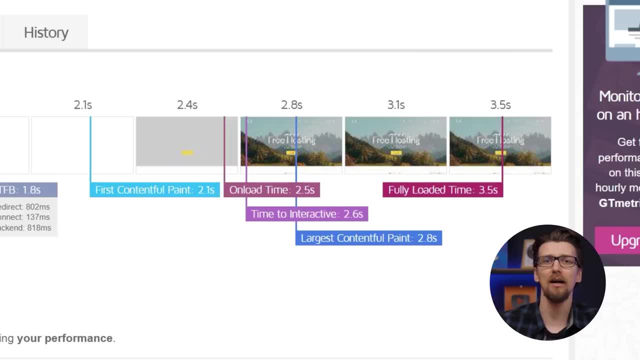 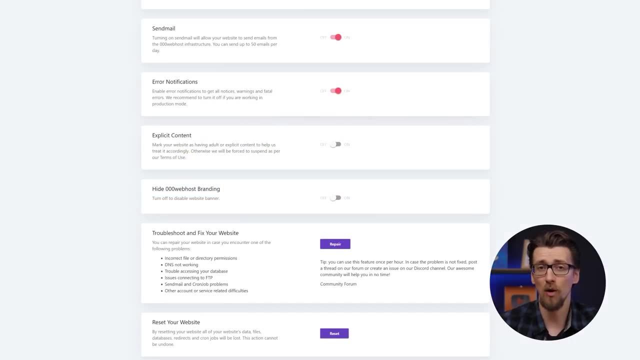 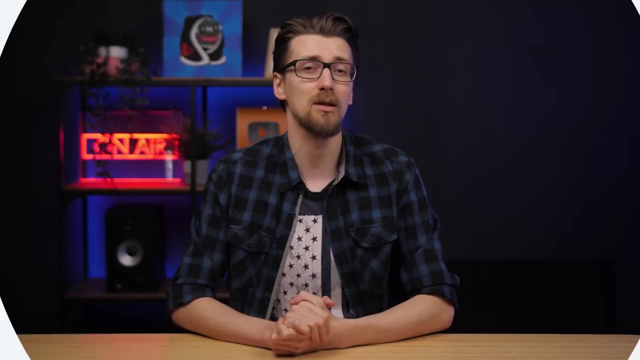 The performance is okay, fully loading a much lighter site that I tested with other providers in 3.5 seconds. Now the interesting part about 000webhosting is that they do allow you to host adult content, while most- even paid- providers, don't. 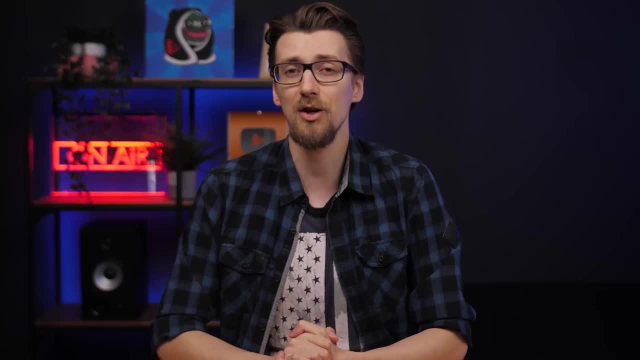 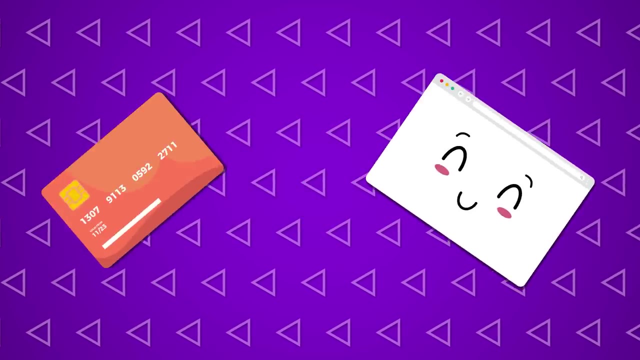 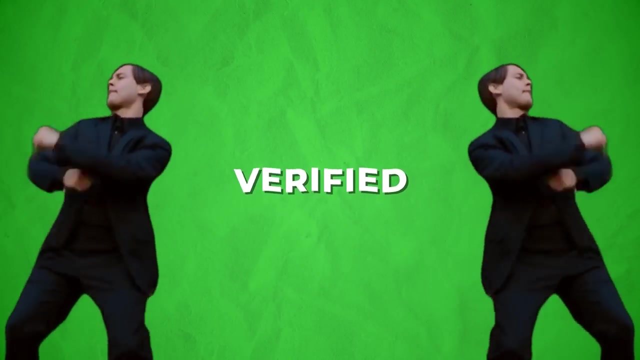 However, the 300 megabytes storage limitation really, really, really, really hurts you. here You can't do much more than a light site, but again, no credit card or payments are required and you can get started within minutes because the verification is automatic. 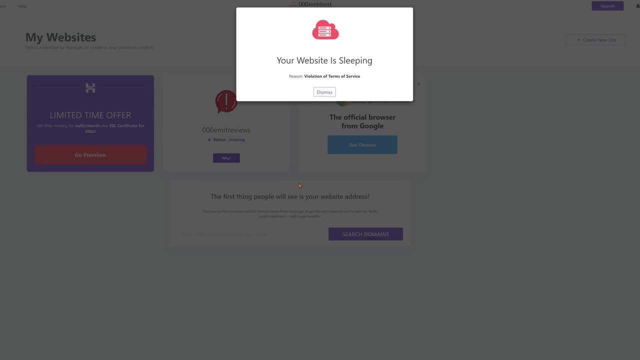 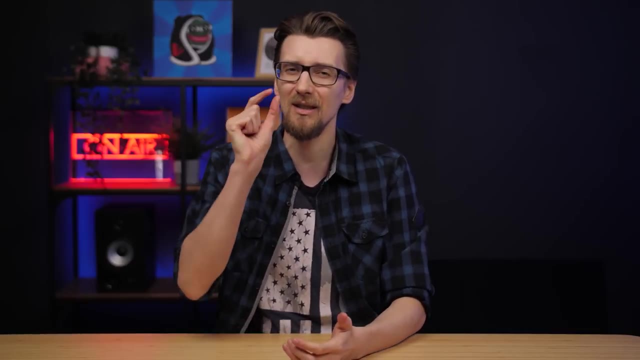 However, I did have my 000webhost website deleted in the past without absolutely any warnings, by accidentally going over the storage limits just by a tad bit. There are no warnings that you're about to go over and they just wipe everything off your server. 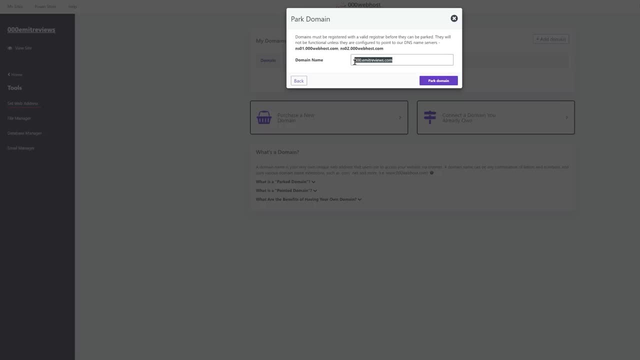 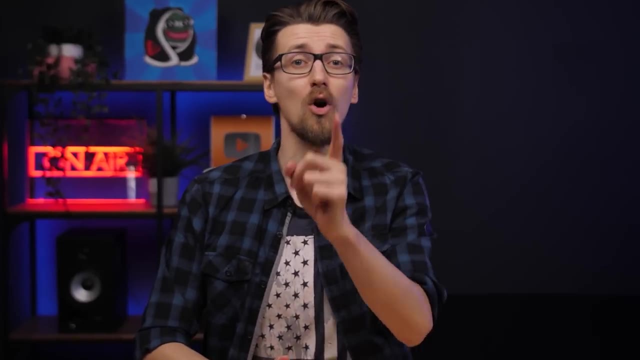 and you're done with your experience. For simple sites, I'd say this works quite well. You can even add a free domain here from Freenum. but for a complex site there's a better way, And I want to talk about that better way. 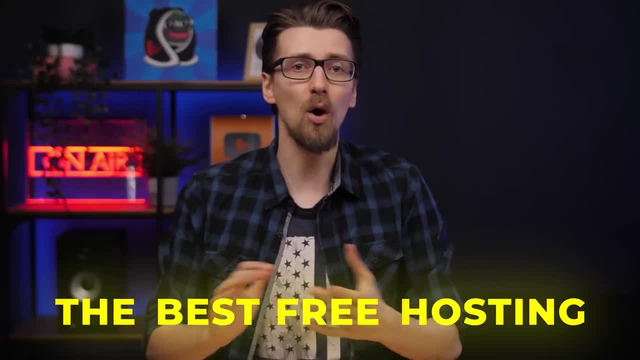 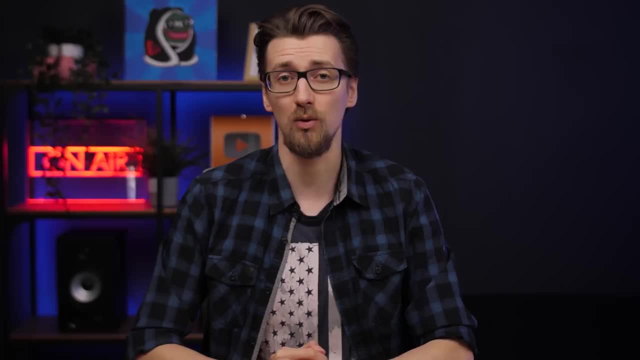 because it's what I consider to be the best free hosting option available. In most cases it's even better than some of the paid plans I've encountered, but it does take a little bit of technical knowledge to get started. I'm talking about free virtual private server on oraclecom. 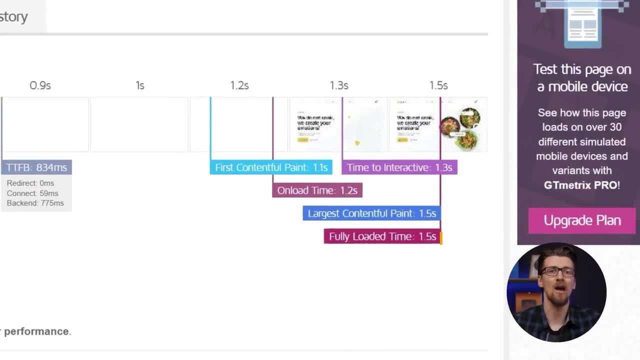 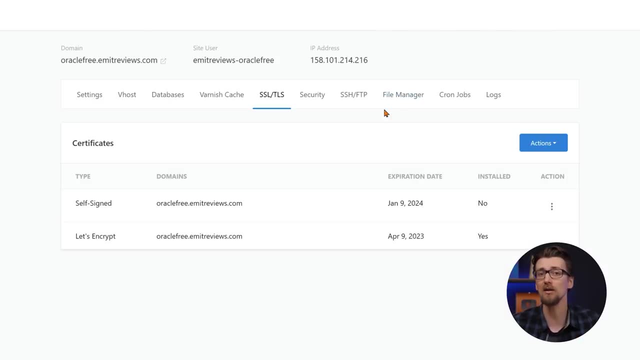 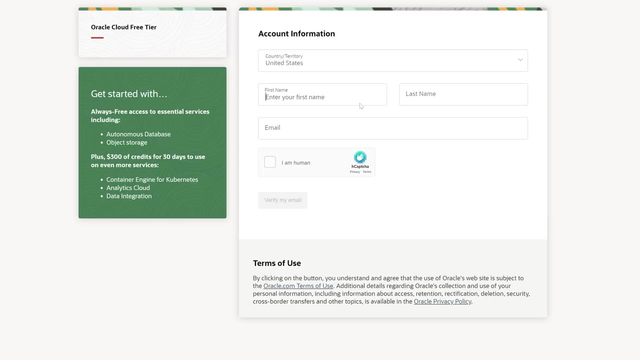 I've actually set up my testing website here. and look at this: 1.5 seconds load time and the website has every premium feature, like a custom domain, SSL certificates, file managers, auto installers and even email. The way this actually works is you apply for a free server. 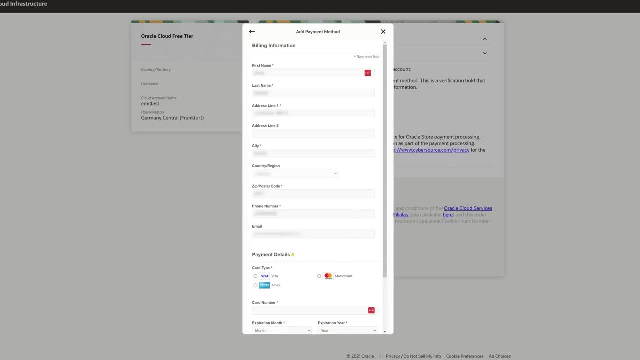 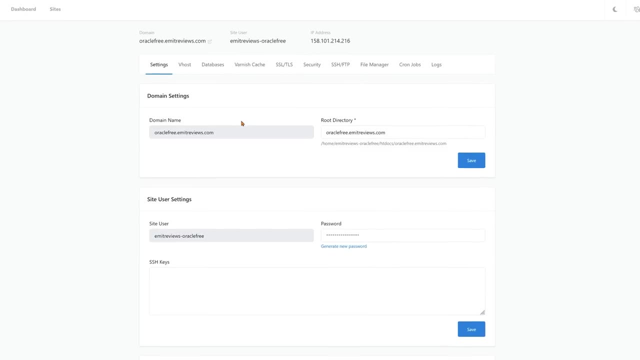 You'll have to have a valid credit card for that work and you will get charged like $1 for verification, but you'll get that back. Then you use that server to host your website and your control. That way you don't have to worry about. 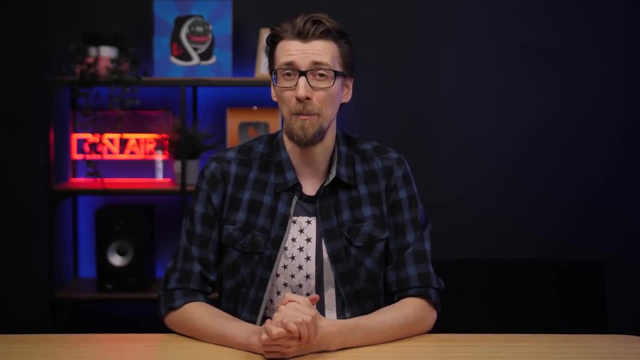 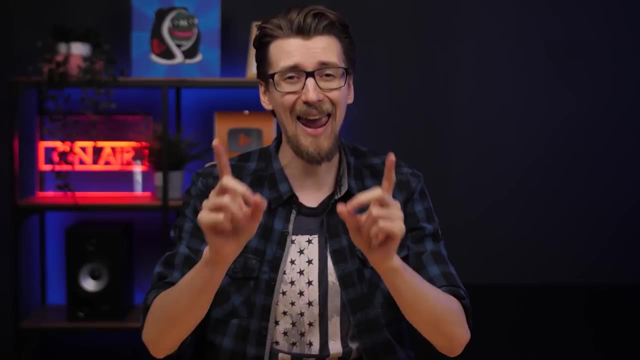 having to do the same thing over and over again. You can just go to your website and click on the panel. It's a bit technical, but I do have a tutorial how to do everything step by step that you can find right here. But before you go ahead and do that, 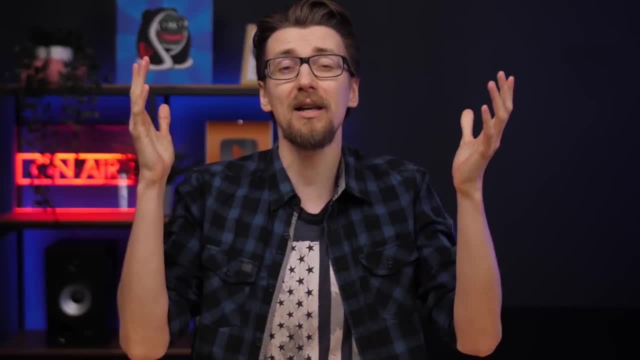 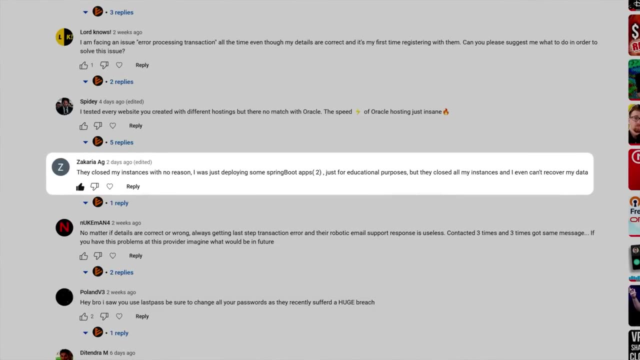 remember that any one of these providers can, and probably will, delete your website at some point, Even oraclecom, which is like a $230 billion company, For example. here you can delete a server with everything on it without a way to recover any of the files.